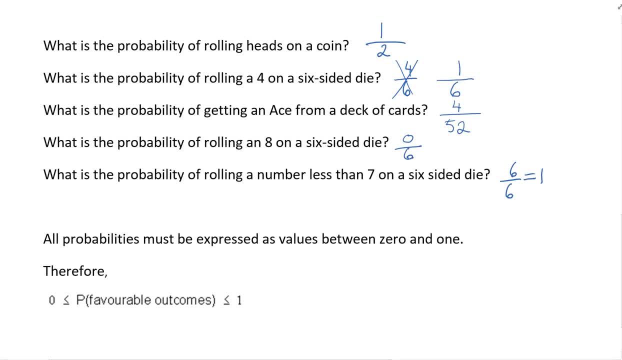 which would be the same as one, and zero out of six is the same as zero. All probabilities: if you look at the probabilities that we just figured out, they must be expressed as values between zero and one. You will never have a negative probability. and so down here this zero. 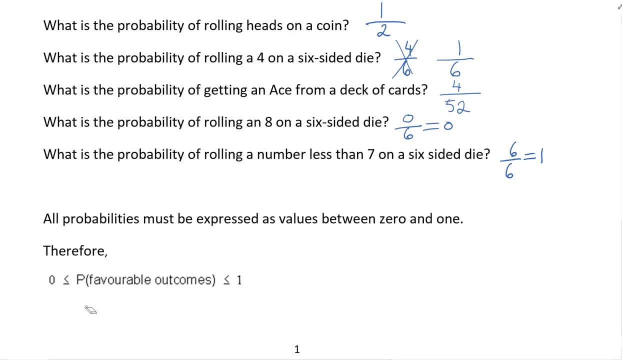 is less than or equal to our favorable outcomes. which is less than or equal to one just means all of our probabilities will be between zero and one, always, Never negative, never greater than one. All right, let's take a look at the next page here. 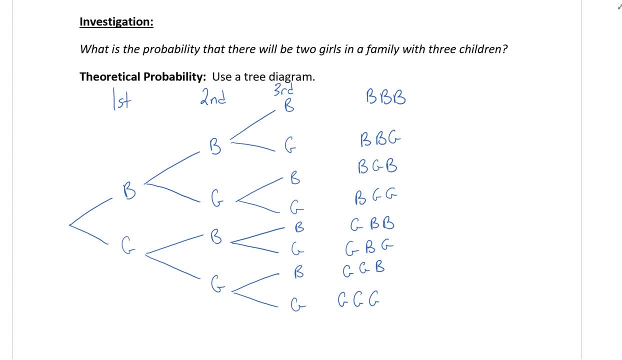 Now this is the start of an investigation that we're going to look at. It says: what is the probability that there will be two girls in a family with three children? Now, we've seen this tree diagram before, so I've just wrote it. written it out. We've got our first child. could be a boy. 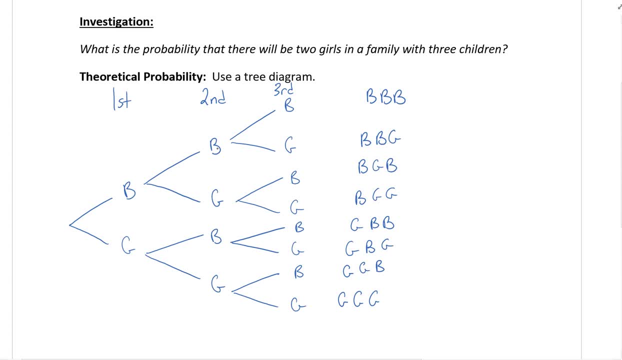 or a girl, the second child. if the first one's a boy, the second child could be a boy or a girl. if the first one's a girl, could be a boy or a girl, and so on, and I've listed out all eight outcomes. Now the question is: what is the probability that there'll be two girls? So I'm going to look at all. 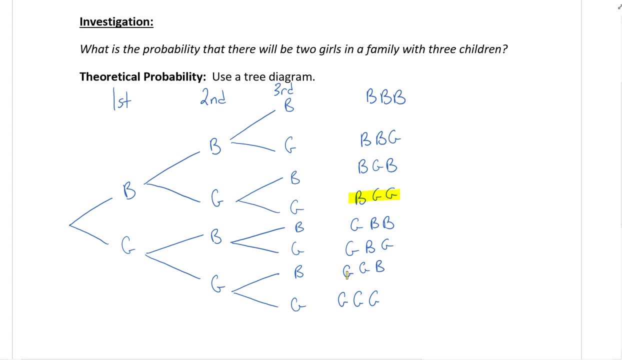 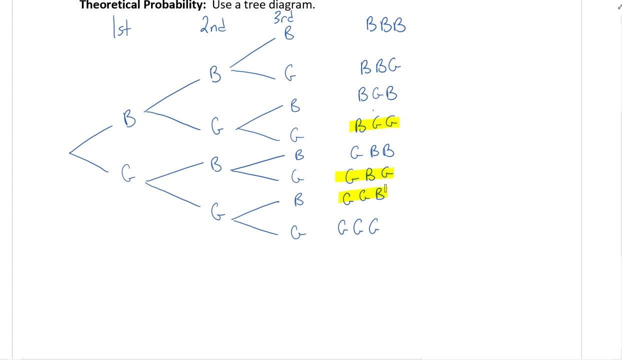 outcomes that have two girls. so there's one, here's another one, and then there's one more. All the rest of these have either more or less than two girls. So how would we write this out as a probability? Well, the probability of a family having two girls out of three children. 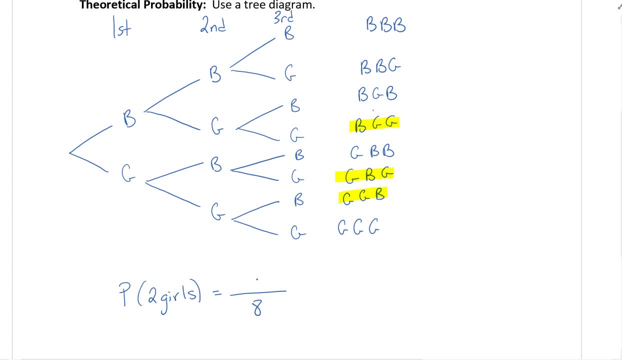 well, the total number of outcomes was eight and we have three out of a possible eight. Now you can write it out as a probability or, if you want, you can write it out as a decimal: 0.0, not 0.0, 0.375. or you can write it out as a. 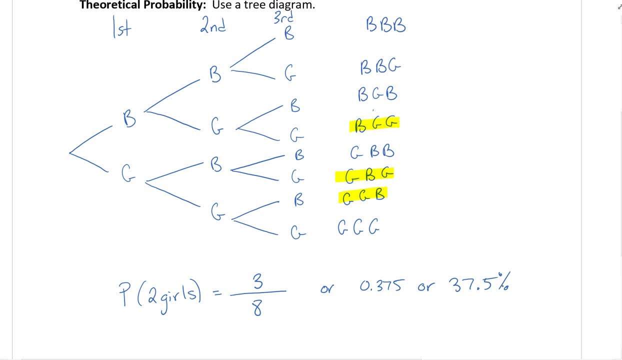 percent, 37.5 percent- Those are all the same representation. Often we'll talk about probability more as a decimal or as a fraction, but there's nothing wrong with a percent as well, and you'll see that coming up over and over again. Now we've done this. this would be the theoretical probability. 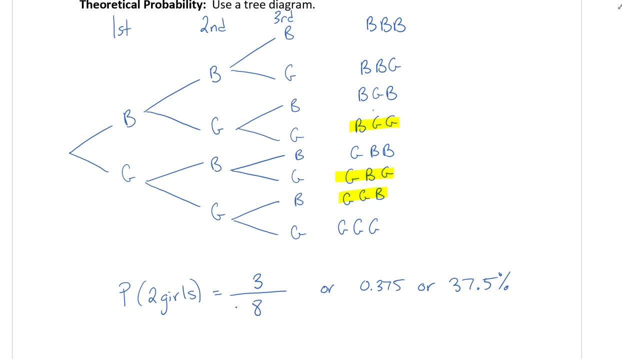 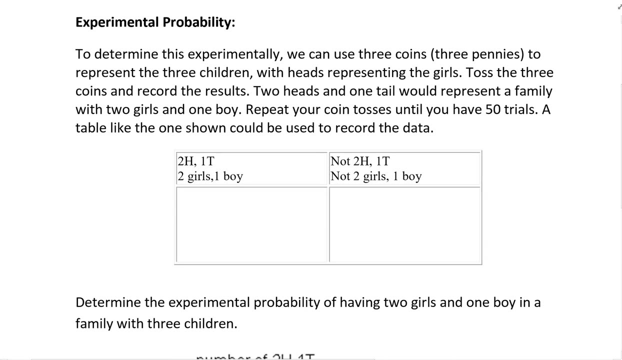 right, this is what we um. what is going to happen Now in terms of an experiment, though? we're not going to, I mean, make people have babies. so we're going to do an experiment here where we're going to use coins, and we'll do this. 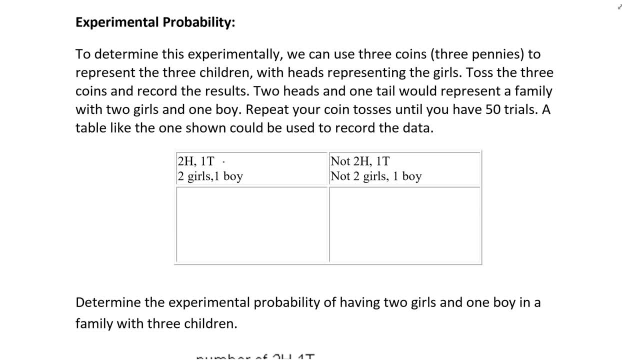 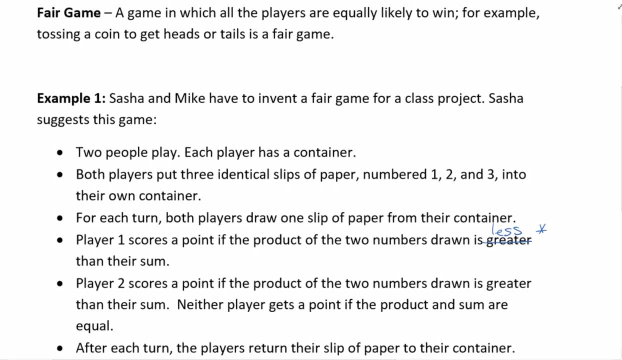 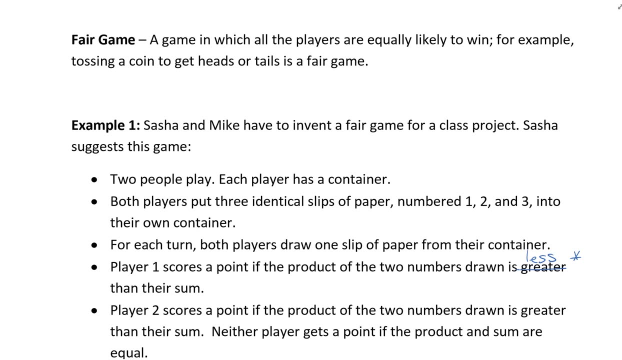 in class and see how close we can get to the probability that we want. One of the definitions that's going to come up over and over again is this idea of a fair game, and that has to do with odds and probabilities as well. Now, a fair game is a game where you can do a fair game, and it's going. 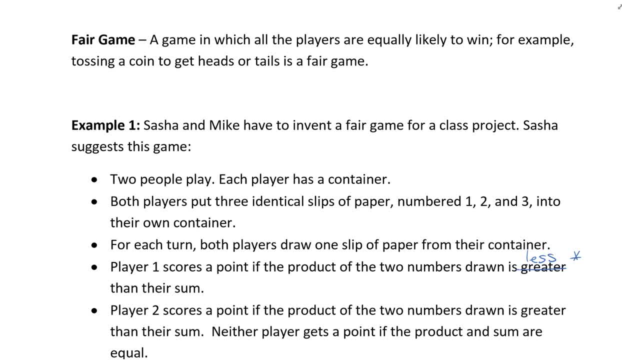 is a game in which all the players are equally likely to win. for example, tossing a coin to get heads or tails is a fair game. why is that? because you have an equal chance of getting a probability of heads and a probability of tails. those are equal probabilities. so here's a game that we go. 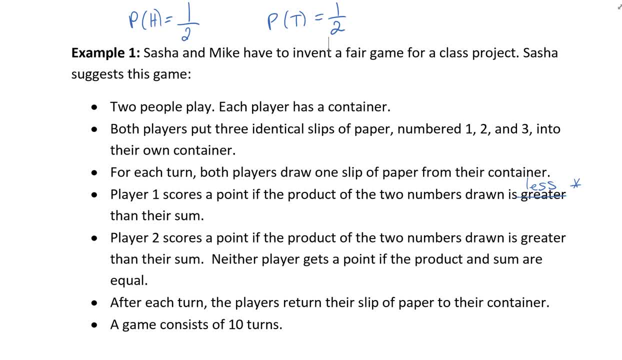 through. we're going to read through this and decide: is this a fair game or is this not a fair game, and we're going to use the probabilities to help us decide. so it says: Sasha and Mike have to invent a fair game for a class project. Sasha suggests this game. two people play each player. 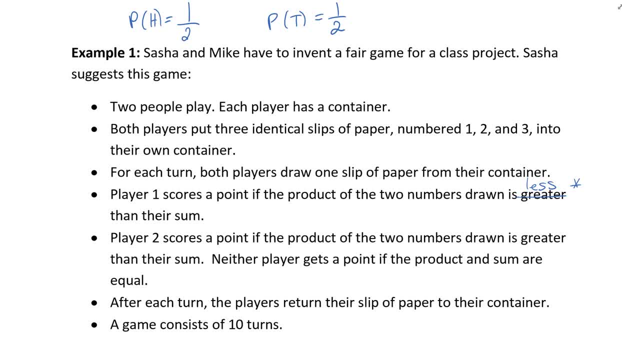 has a container. both players put three identical slips of paper, numbered one, two and three, into their own container. for each turn, both players draw one slip of paper from their container. player one scores a point of the product of two numbers drawn is less than one. player two scores a point of the product of their two numbers drawn is greater than their sum. neither. 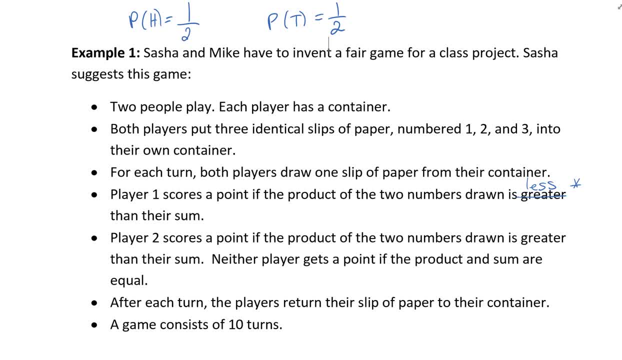 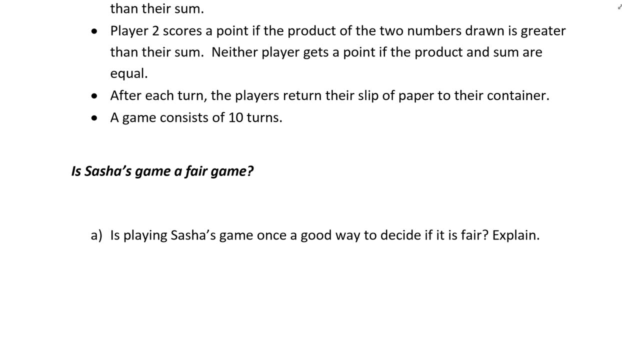 player gets a point if the product and sum are equal. after each turn, the players return their slip of paper to their container. a game consists of ten turns. is Sasha's game a fair game? well, is playing Sasha's game once a good way to decide if it's fair? well, no, because if we only played, 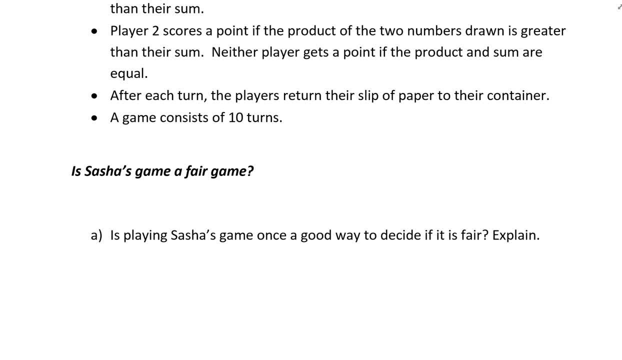 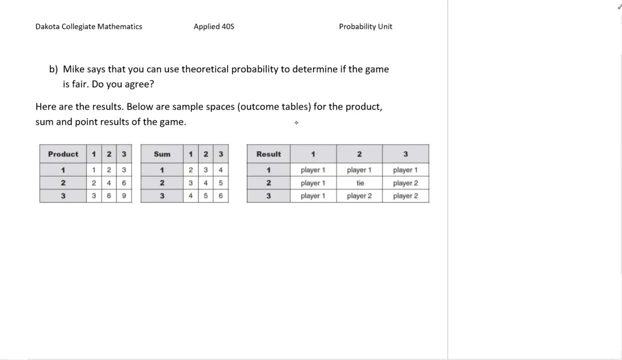 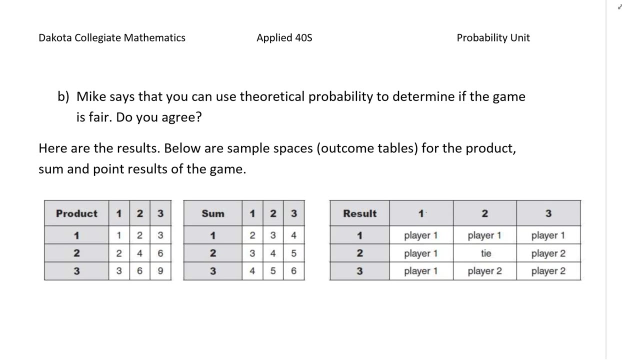 it once. we're not generating an element of a fair game. we're only generating an element of a fair game- data to draw any conclusions right. so once is not enough to get accurate results. Mike says that you can use theoretical probability to determine if the game is fair. do you agree? well, let's have a. 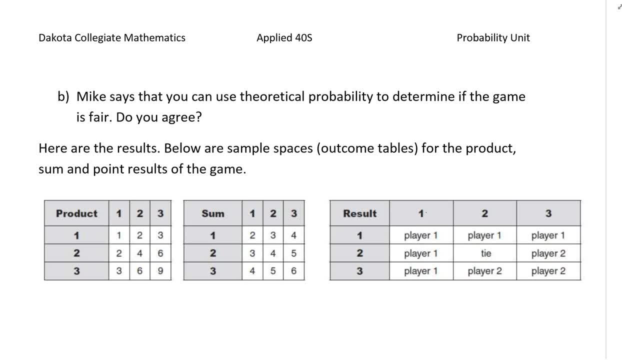 look, it says here the results. below is a sample space for the product, the sum and point results of the game. so if we look here that slip of paper, one and one, when you multiply them together you get a one. when you add them together, you get a two and you get a one. so it's a good idea to have a. 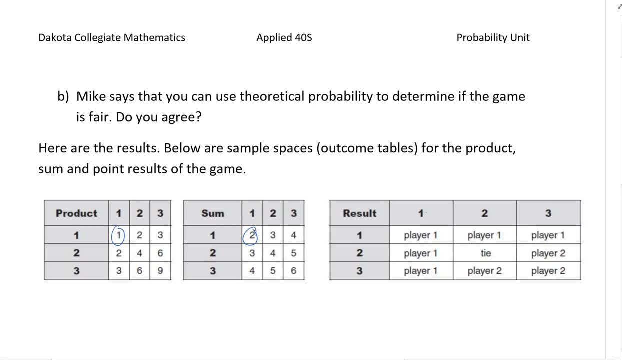 add them together, you get a two. So that's what they're looking at. So if the product is a one and the sum is a one, then player one wins, right. So here, if we look at two and two, that gives you a four and a four and that's a tie. So nobody gets any points. Here we've got. 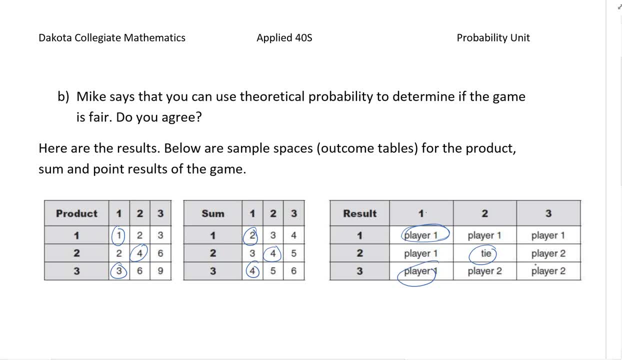 a three and a four and player one wins. So the only way player two can win is here. this is one of the instances with a six and a five, because the product of three and two is greater than the sum of three and two. So that's how the game works. just to see it played out. So let's figure. 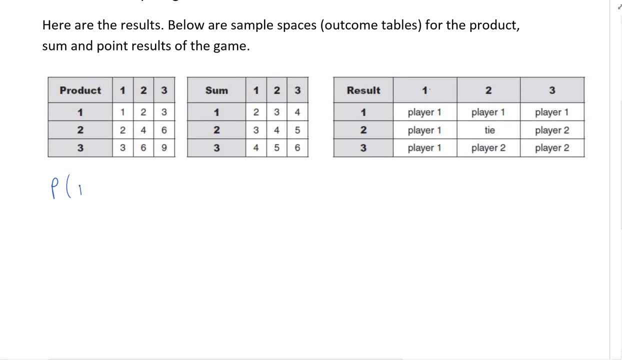 out the probabilities: the probability of player one winning, And let's figure out the probability of player two winning, And then, to make it more complete, we should probably also get the probability of getting a tie. So we can see what all those probabilities are. So, probability of player one winning: we can see. if this is our sample space, 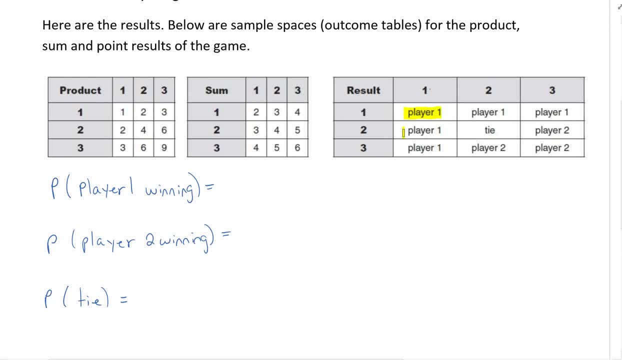 right. Player one wins 123.. Four, five times, So that would be five out of how many. we've got a total of nine different outcomes. And then player two winning would be three out of nine and then a tie as our. 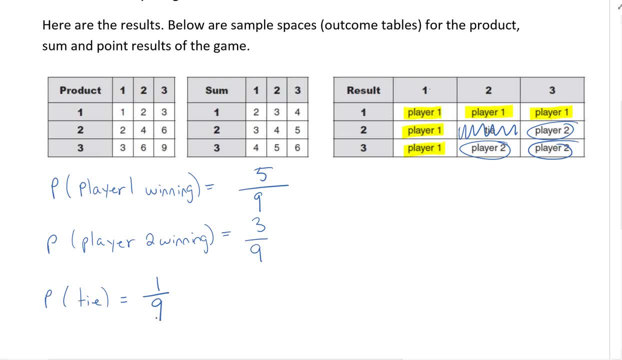 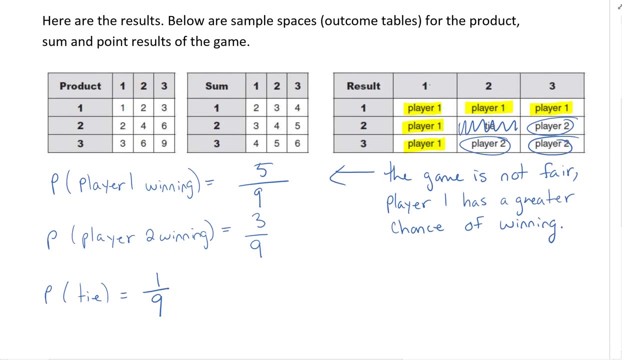 last one here, And that would be one out of nine. So you can see here that the game is not fair and player one has a greater chance of winning. So to answer the question above here it says: Do you agree? Well, yes, we do agree. we use the theoretical probabilities And